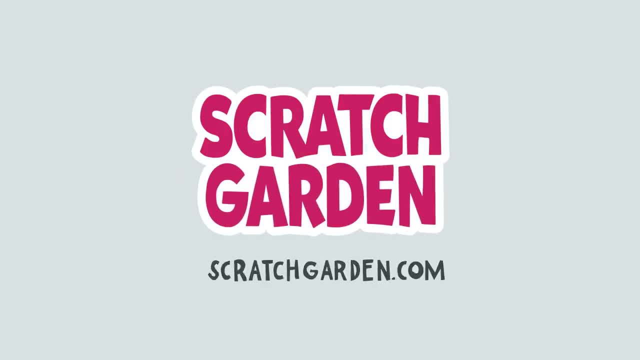 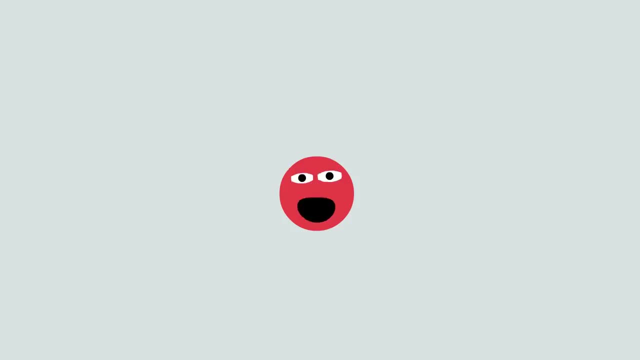 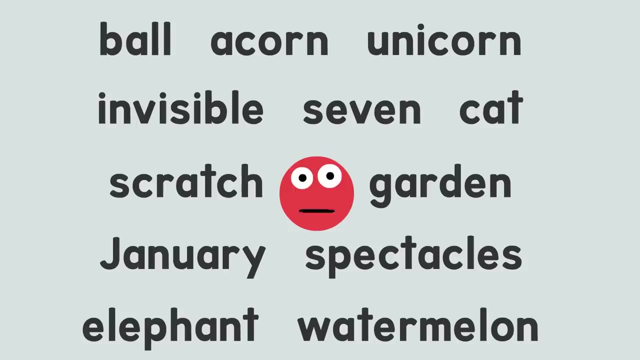 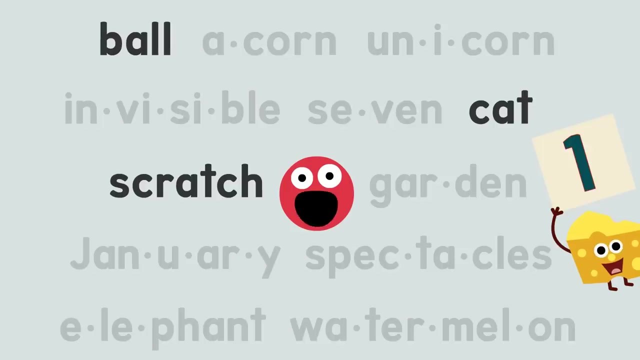 Hi, Okay, everybody. The English language has many words like this, So many words, And every word can be split into parts. We call these parts syllables. A word could have one or two or three or four or even more syllables Syllables. Could a word have one million syllables? 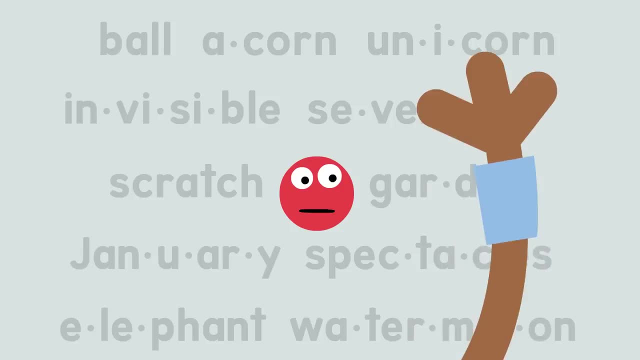 No, that is too many syllables. What about four syllables? Yes, I already said that. Ha No more questions. Anyway, a syllable is like a beat. Do you know what a beat is? Drummer, please play a beat. 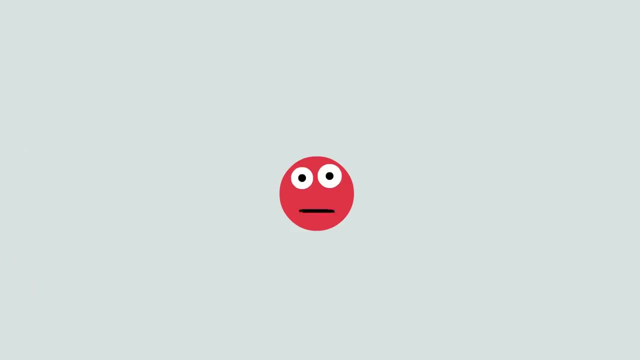 Thank you, That is a good beat. You can make a beat by clapping your hands. Now, get those hands up, Let's practice one beat. Okay, ready, Here we go, Clap Ha-ha. Now let's try it with some words. We start with the easy ones. 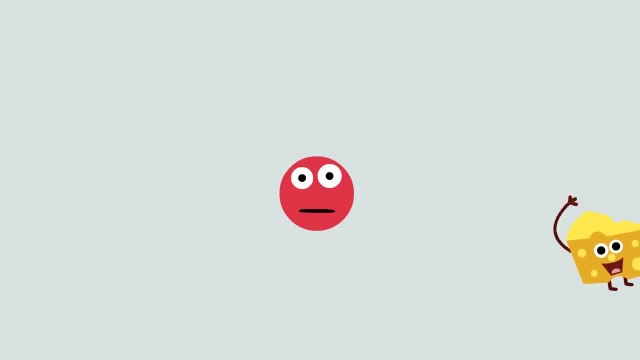 Words with one syllable and therefore one beat. The first word is dog, Dog, Dog. It's a dog. Ha-ha, Good girl. Now everybody clap your hands to make one beat when I say the word dog. Okay, 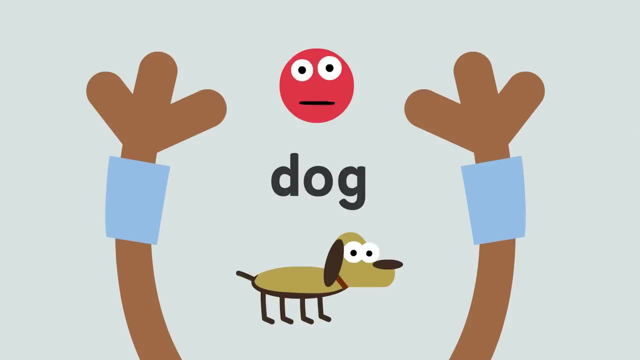 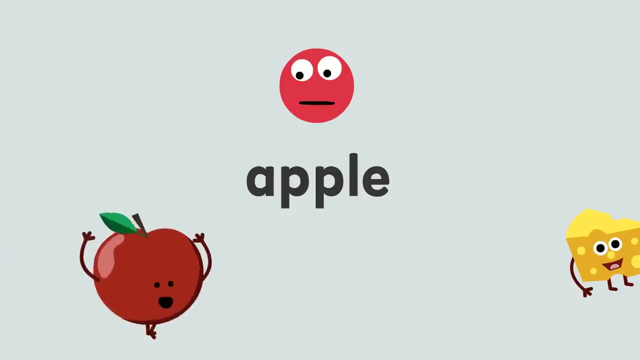 ready, Here we go. Dog, Dog, Dog, Dog, Dog Dog. Hey, Good job. Next we will try a word with two syllables: Apple, Apple, Apple, Apple. I said Apple. Huh, thank you. 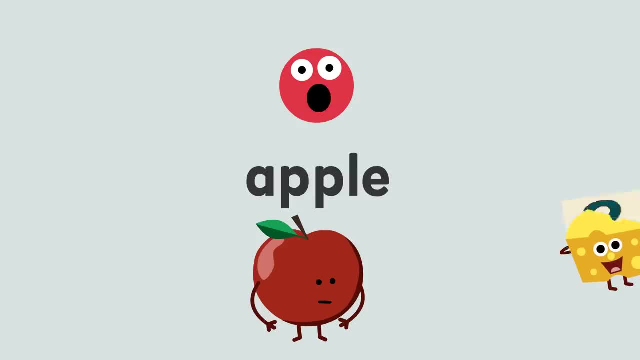 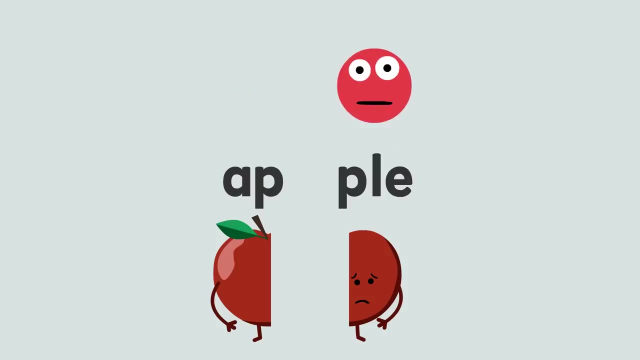 The word apple has two syllables and therefore two beats. It's kind of like it's split into two parts like this: The first part is app and the second part is pull. Now everybody clap your hands and make a beat when I say each part of the word apple. 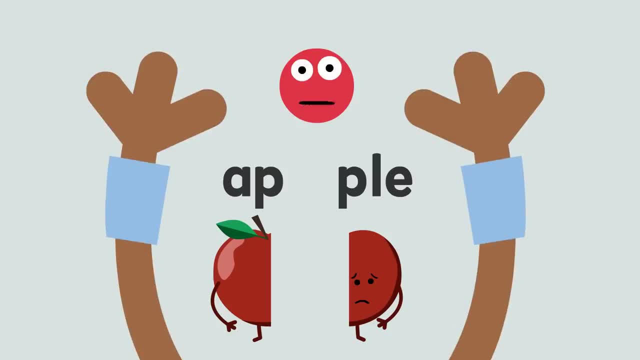 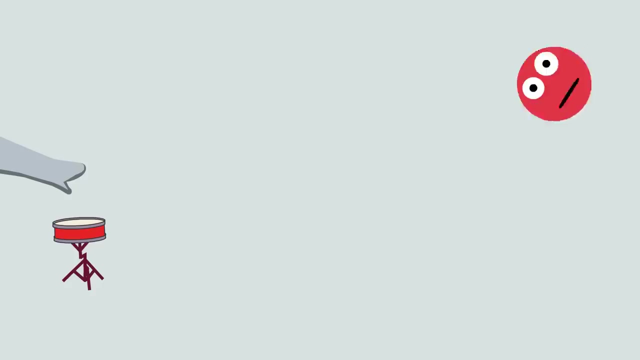 Okay, ready, Here we go. App-pull, App-pull, App-pull, App-pull, App-pull, App-pull. Yeah, You're doing great. Next we will try a word with three syllables: Ladybug. 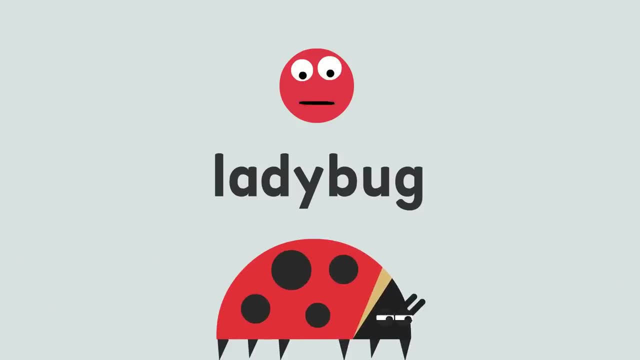 Ladybug. I said ladybug. Wow, that is a big ladybug. The word ladybug has three syllables and therefore three beats. It's kind of like it is split into three parts. The first part is lay, the second is dee and the third part is a bug. 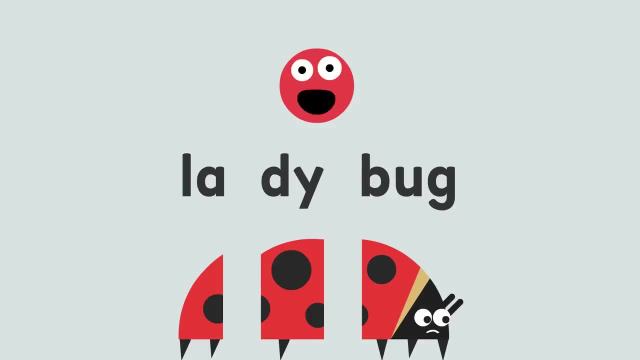 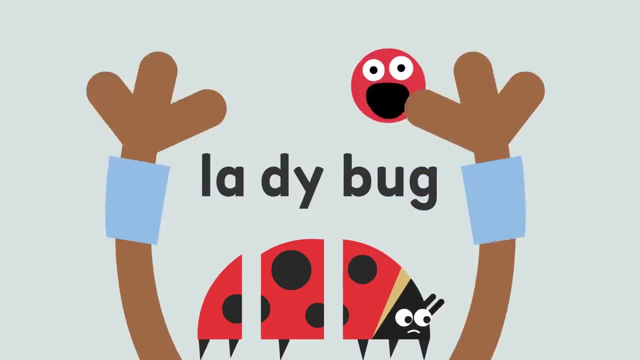 Now everybody clap your hands and make a beat when I say each part of the word ladybug. Okay, ready, Here we go. Lay-dee-bug, Lay-dee-bug, Lay-dee-bug, Lay-dee-bug. 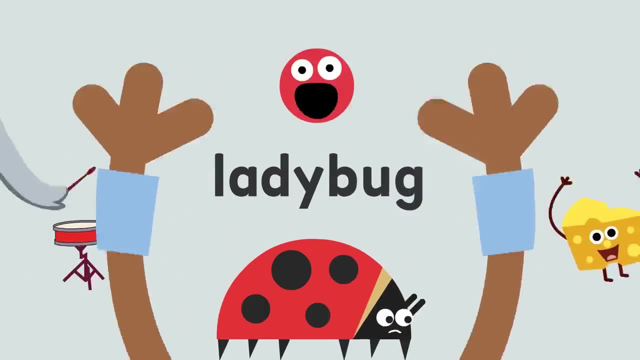 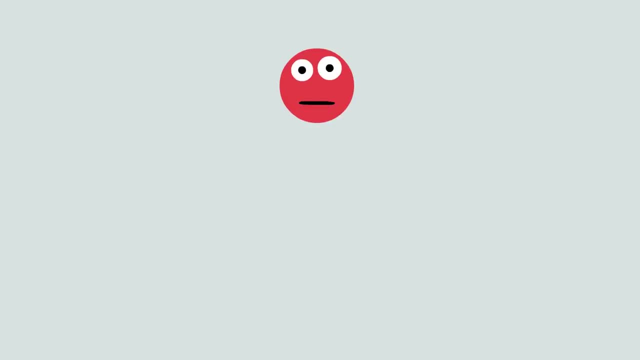 Lay-dee-bug, Ladybug, Good job. And finally, we try a word with four syllables: Salamander, Salamander, Salamander, Salamander. It's a salamander, Hooray. 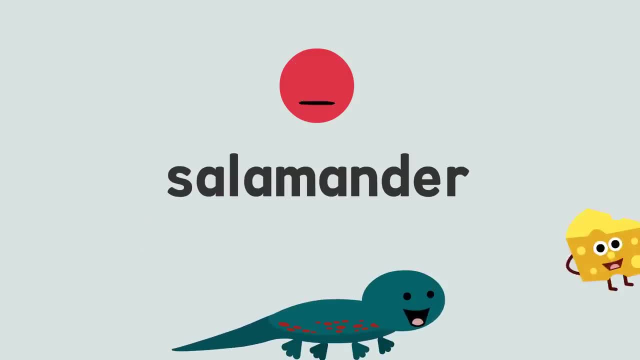 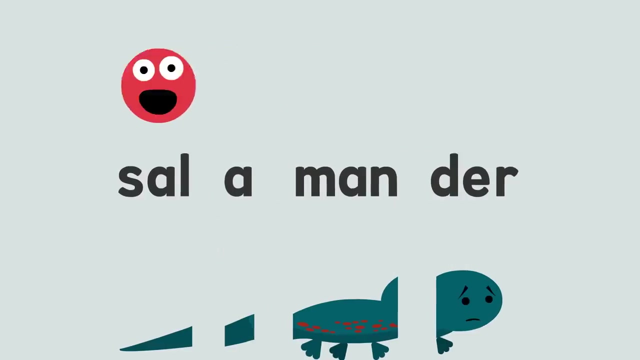 Ho Hi salamander. The word salamander has four syllables and therefore four beats. It's kind of like it is split into four parts. Ow, The first part is sal, the second part is a, the third part is man and the last is der. 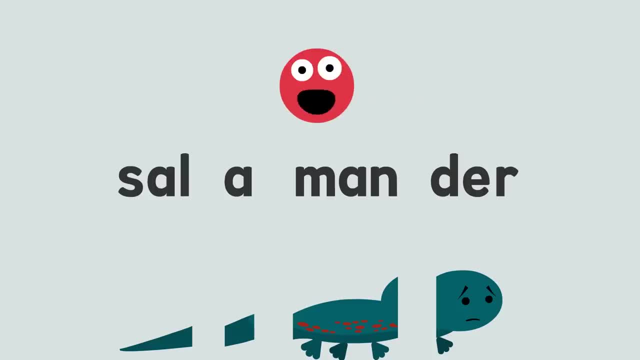 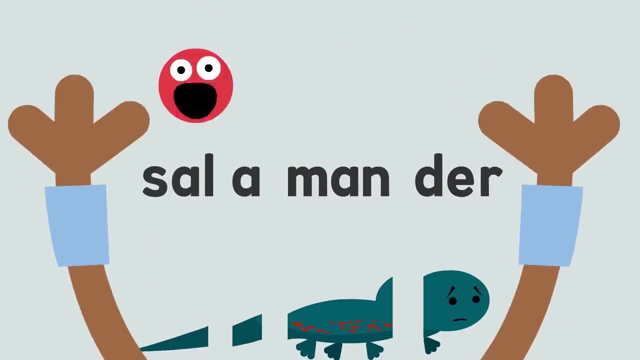 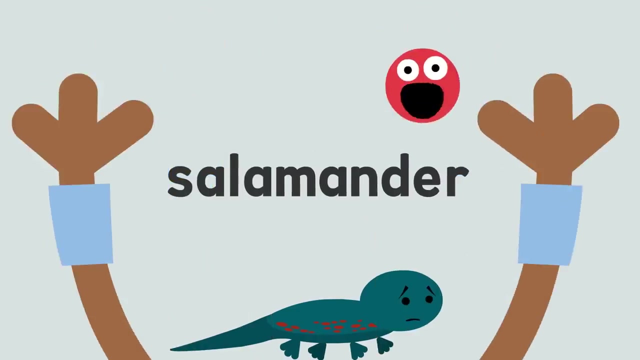 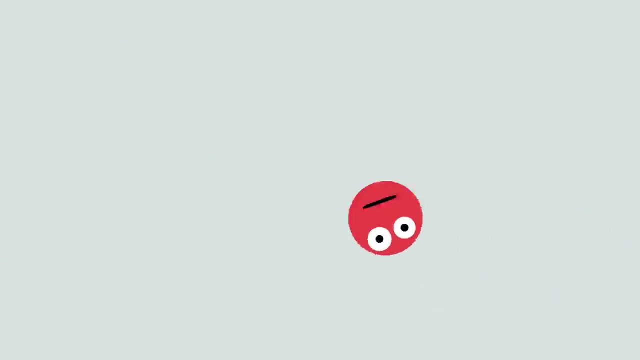